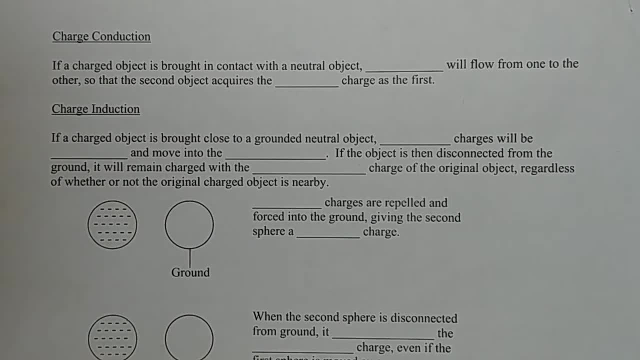 causes the electrons that are kind of knocked loose to be attracted to whichever one of the two materials is most inclined to become electropositive, electronegative, I mean whichever one has the greater tendency to take on greater electrons. So that's sort of a common way of 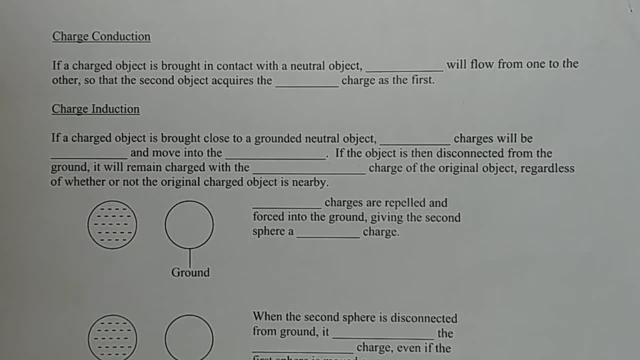 causing static electricity is to rub two objects together and one of them gains electrons and the other one loses electrons. So now we've done that and we have some charged particles. What if we want to transfer that charge to another object? Well, if you have an object with extra electrons, 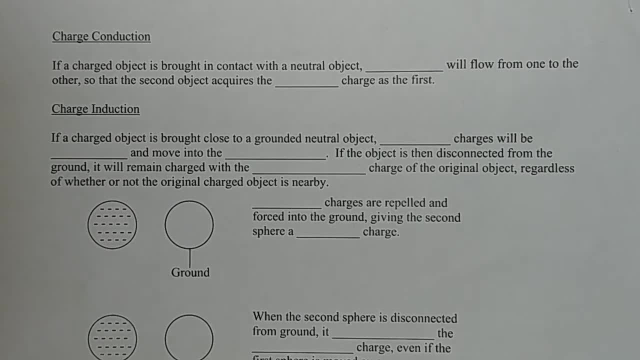 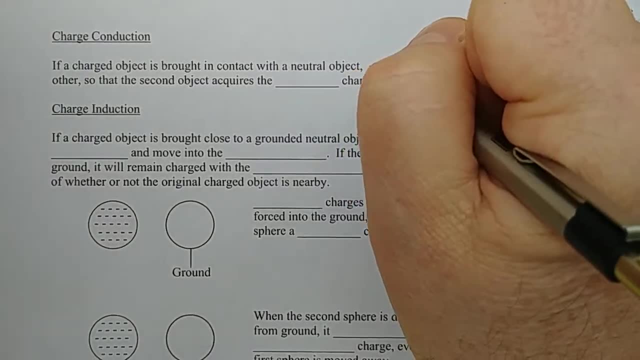 and you want to charge it. you can do that. You can do that by using a charge. You can do that if you touch it to another object so that the electrons can float from one to the other. Some of the electrons will flow from that object to the other object And, as a result, if the first one had 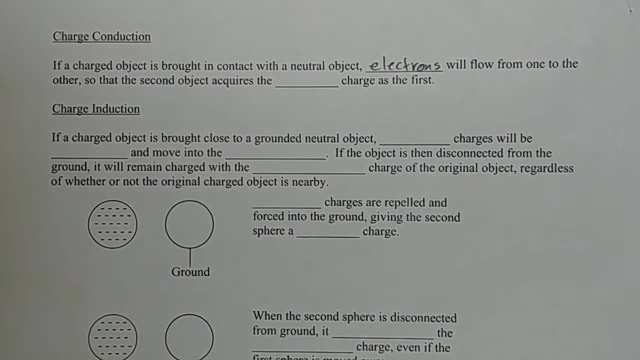 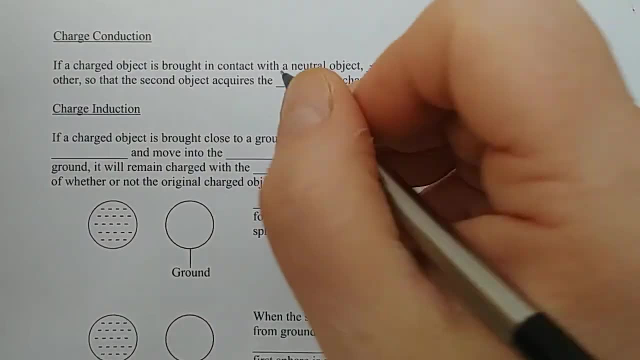 extra electrons and now some of those extra electrons have now flowed to the second one- not all of them, just some of them- then what happens is the second one will also have a negative charge, So it will end up with the same charge. So if you have a bunch of extra electrons, 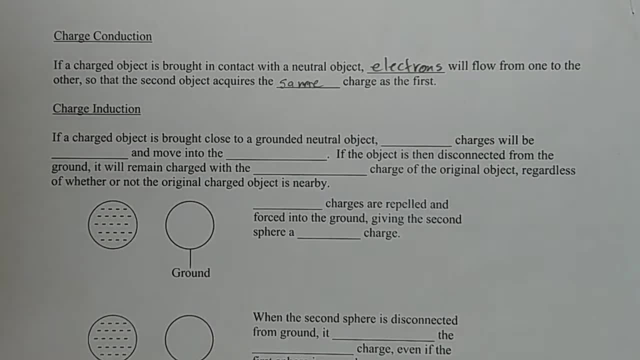 they're kind of repelling each other because they're all negative. They want to get out of there if they can. And if you touch them to another object so that there can be a flow of those electrons, then some of them will flow out Because they're all. 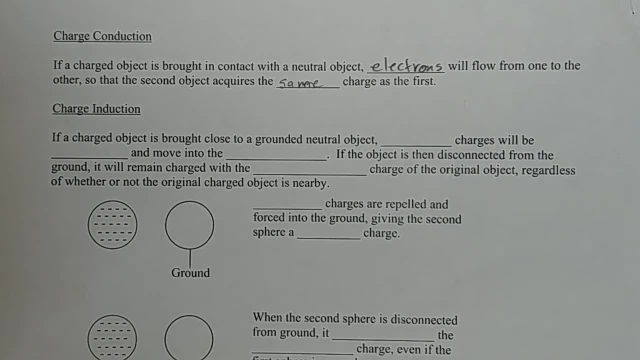 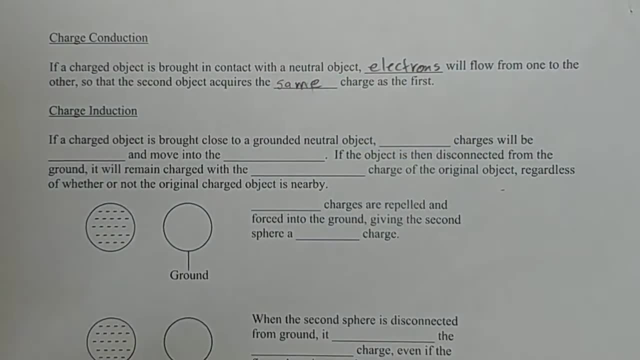 repelling each other. they're trying to sort of spread out as much as possible. and they will spread out among the two objects. So the first one will maintain its negative charge because those electrons aren't all going to travel to the second one. They want to travel, spread out as much as. 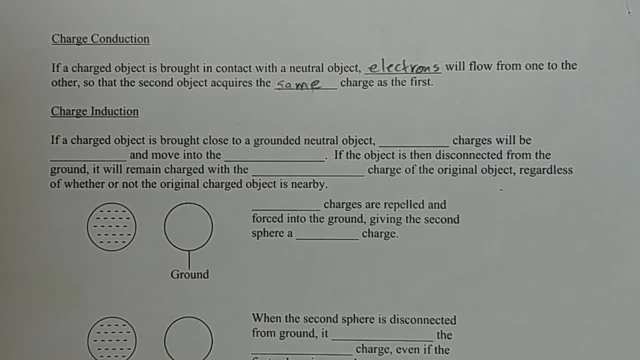 possible. So some of them are going to stay where they are, while other ones go over to the other object. Similarly, if you have an object with extra electrons and you want to charge it, you can do that. Similarly, if you had something that was missing electrons, because it's positively charged. 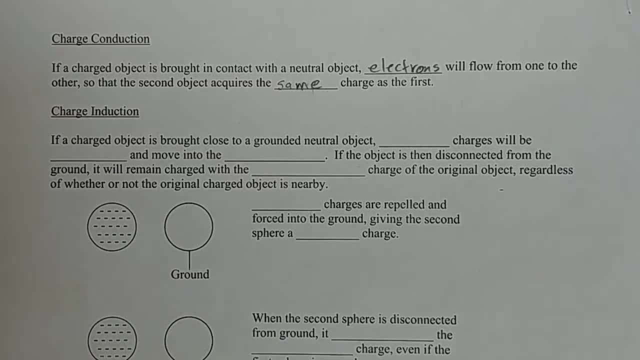 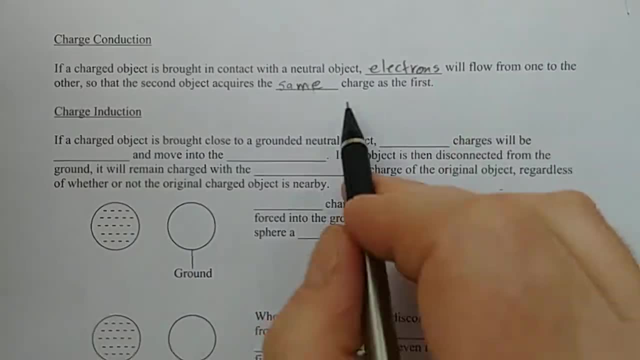 and you touch an object, then what it will do? it will attract electrons from the other object and the other object will become positively charged as well. So basically, conduction causes is simply touching two objects to another, And what that does is it transfers the same charge. 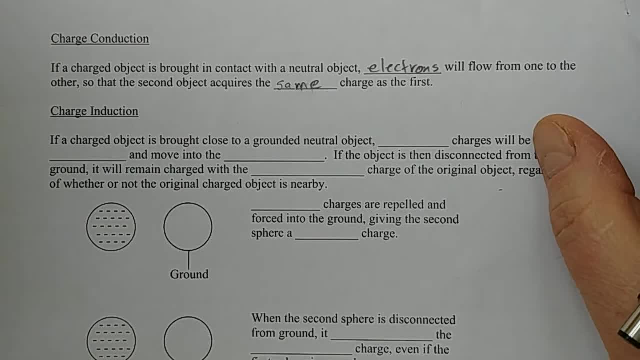 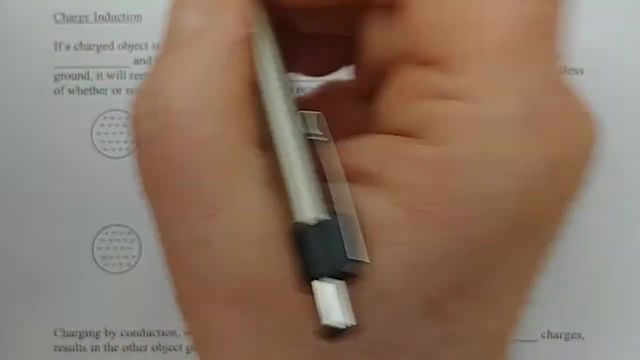 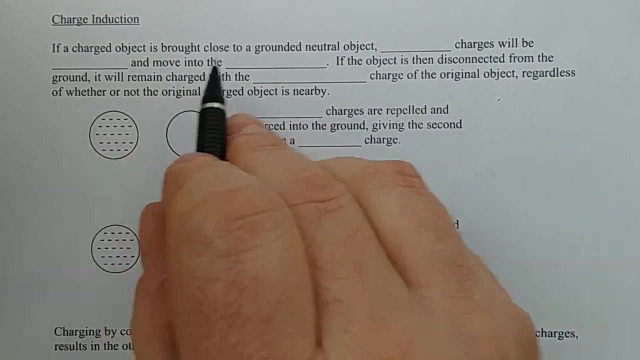 to the second object as the first one had. Now there is another way to charge objects and it is called induction. Induction means without contact Conduction. contact induction means you have no direct contact of them. So what we're going to do here is we're going to take a charged object and we're going to bring 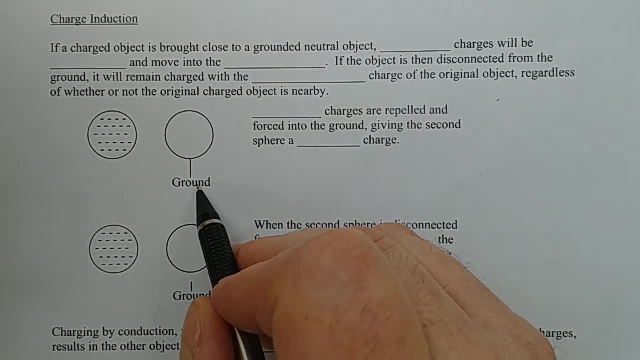 it close to a grounded neutral object. By grounded we mean literally touching the ground, as in touching the earth. Why do we want it to touch the earth? Because the earth is a really, really big object that can very easily gain or lose electrons, no problem at all. 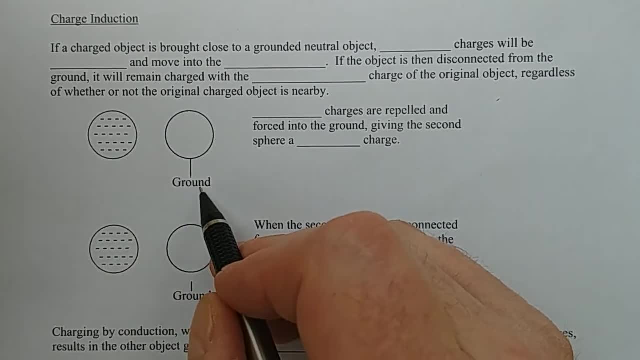 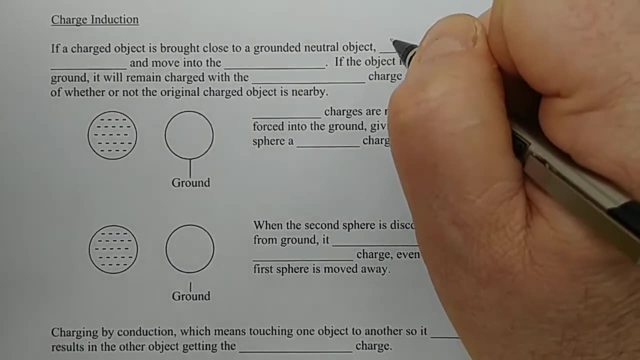 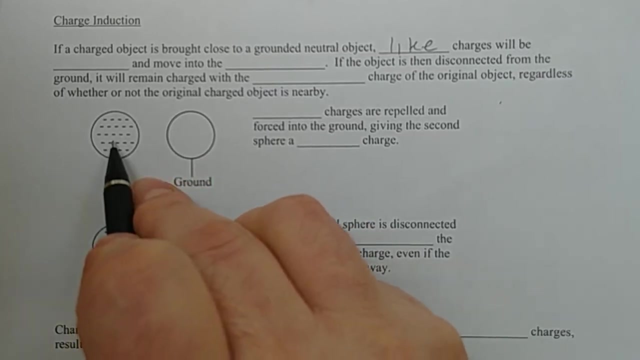 So if we take this negatively charged object and we bring it to this ground, this grounded, neutral object, what's it going to do? Well, like charges, the electrons- in here these are- say this is negativeness. So what's it going to do? 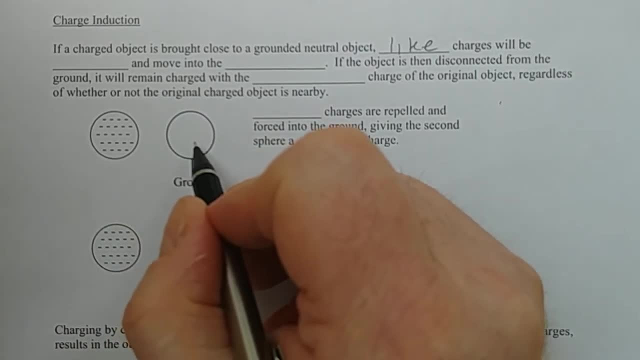 It's going to repel the negative, the electrons, not all of them, just a tiny portion of them, But some of the electrons, because this is going to be pushing on electrons and creating a force on electrons, trying to push them away. these electrons are going to try to get away. 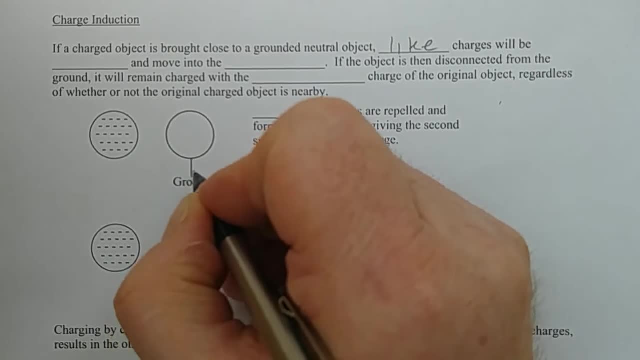 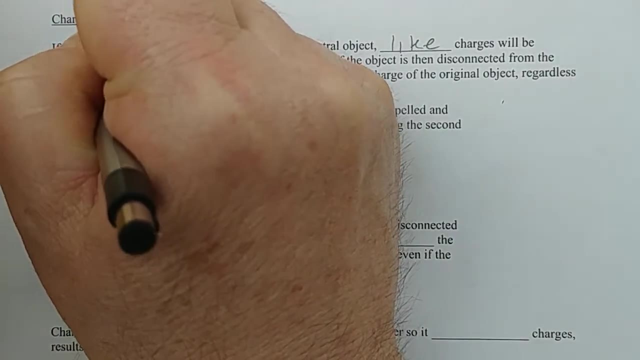 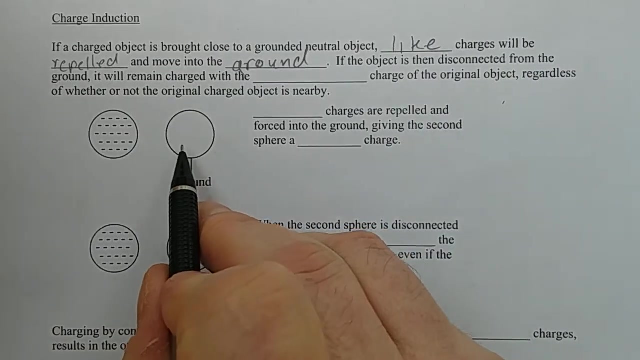 And how are they going to get away? Well, if there's something connecting to the ground, they're actually going to go to the ground and spread throughout the earth, So like charges will be repelled and move into the ground. So here there was a neutral object. 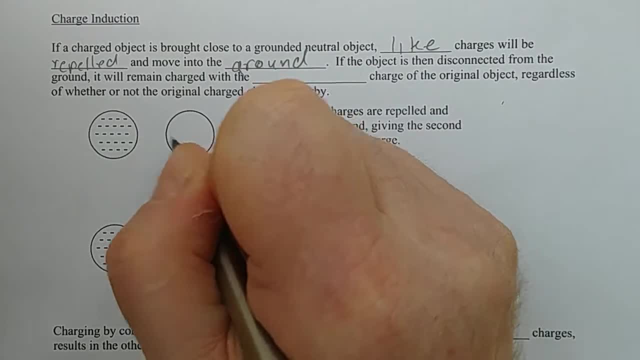 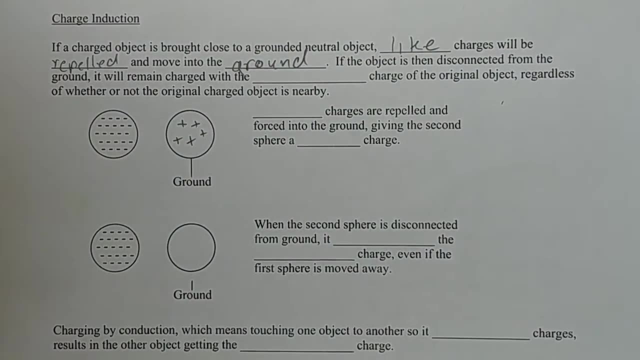 But what have we done? We have repelled negativeness, We've gotten rid of some electrons, We've pushed some electrons out, And so what's going to be left behind is something positiveness. So what happens in this example is that negative? 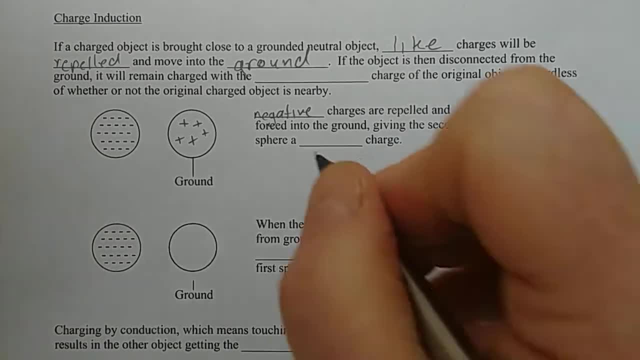 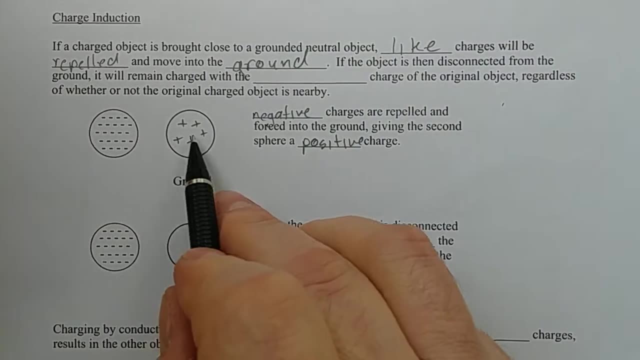 charges are repelled and forced into the ground, giving the sphere a positive charge If the object is then disconnected from the ground. so this had a positive charge And the reason why it had a positive charge: it went from neutral to having a positive charge. 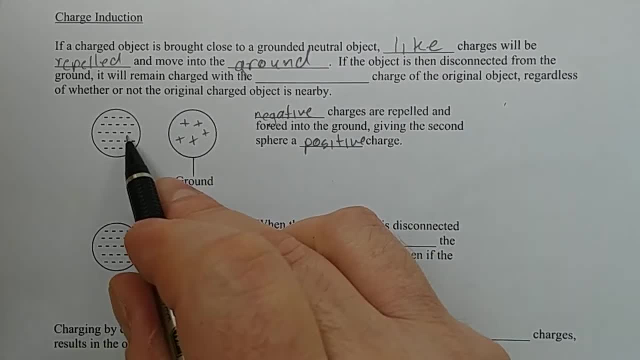 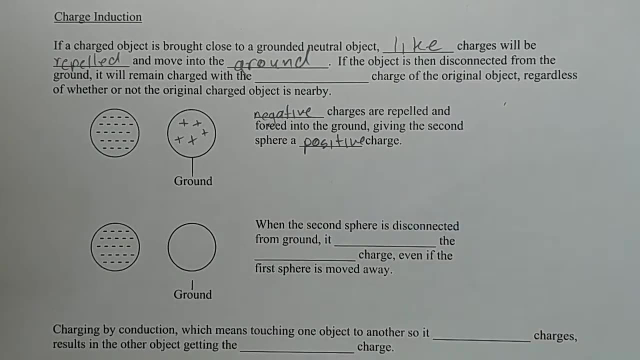 because it was connected to the ground. So there was a way for these electrons- some of the electrons in here that were being repelled by these electrons- could get out of there and go into the ground. But now, if we disconnect it from the ground, what happens?